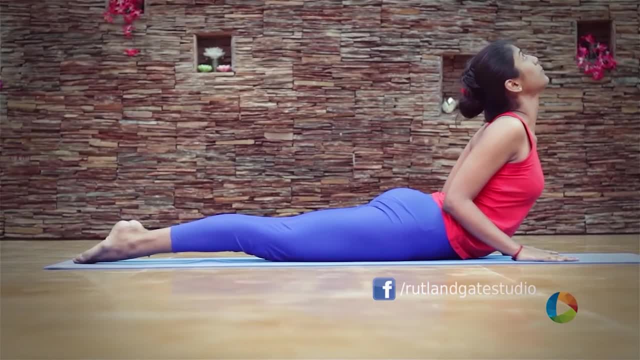 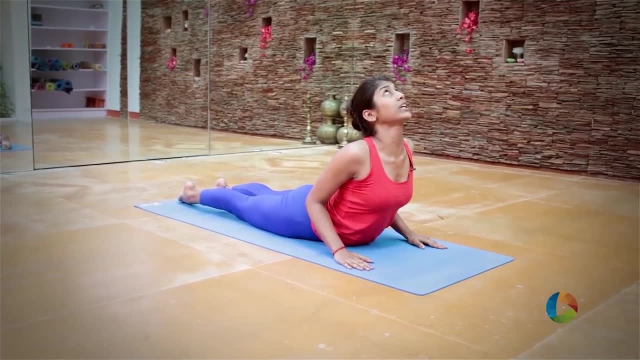 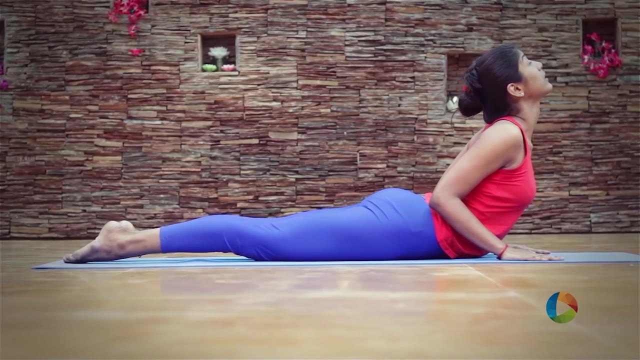 be on the mat. Okay, Lift your chin up, look at the ceiling, Stay here for 5 breaths. When you stay here for 5 breaths, put all your upper body weight on your middle back and strengthen your middle back as much as possible And exhale down. Now we will do one more variation. 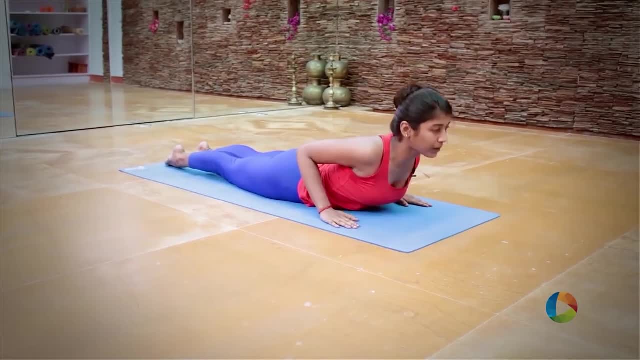 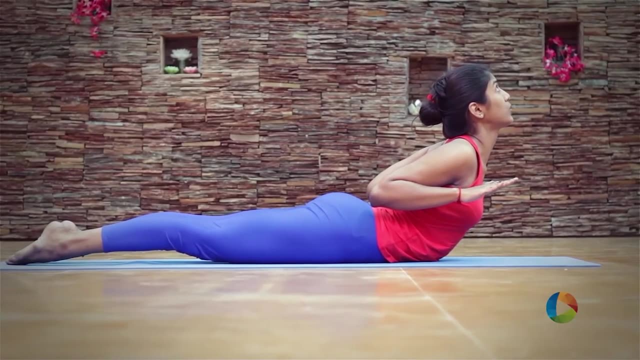 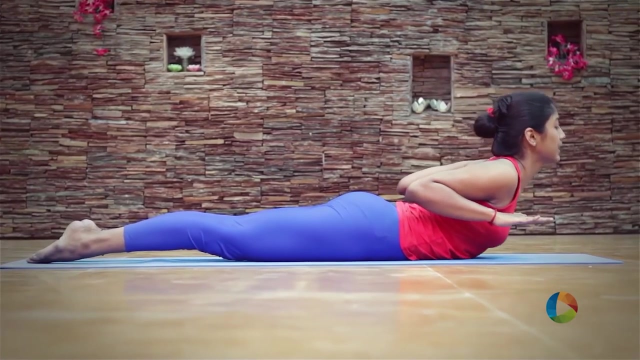 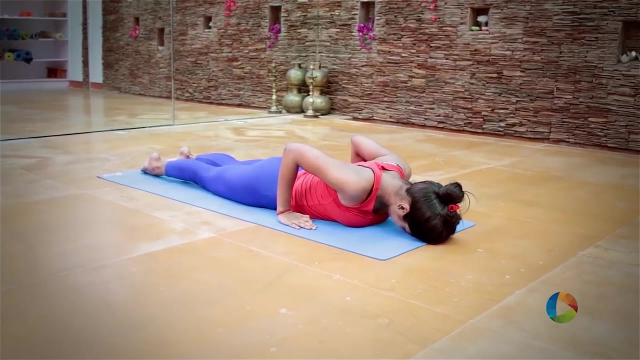 in Bhujangasana The same thing. Inhale and come up such that the navel point touches the mat and gently lift your hands off the mat. Stay here, Shift all the body weight towards your lower back and strengthen your lower back. Exhale down Now. gently place your hands down in between your shoulders. 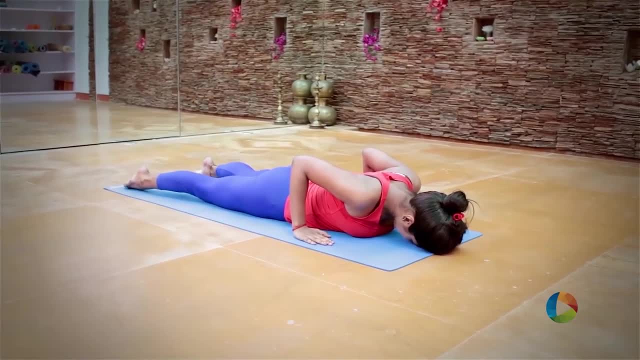 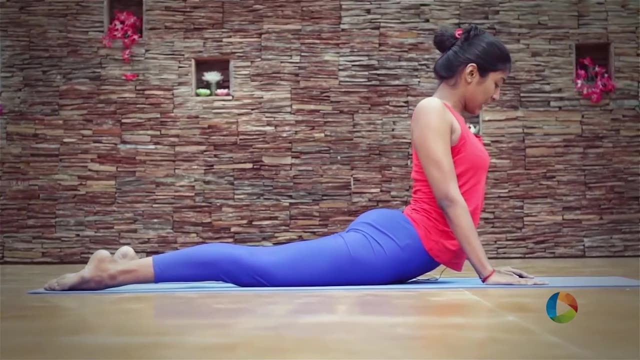 and your pelvic bone. Open your legs slightly out, Inhale and then come up. Now lift your navel above the ground level, Push your pelvic bone down, Procure your pelvic bone down and then, elbows straight, Push the shoulders back. 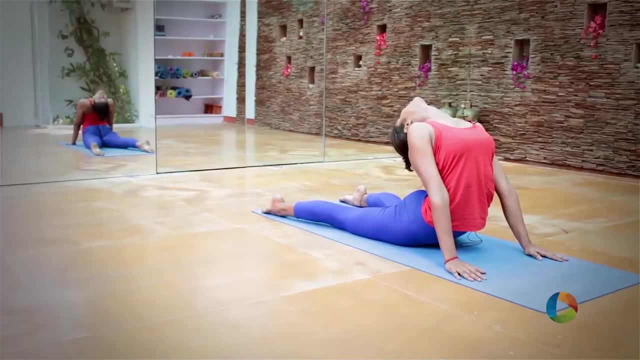 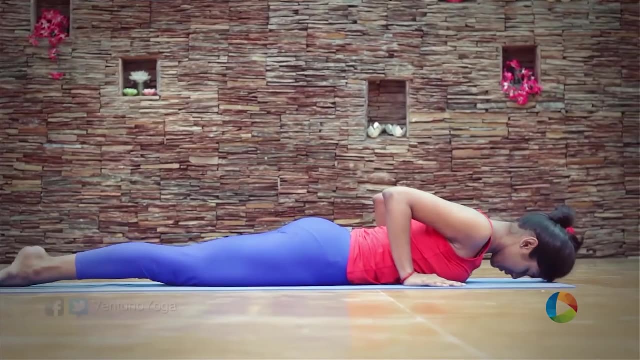 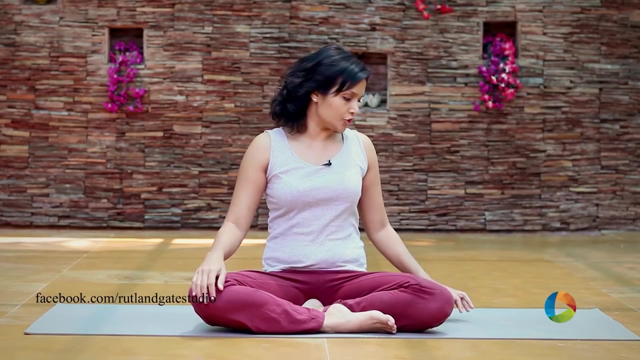 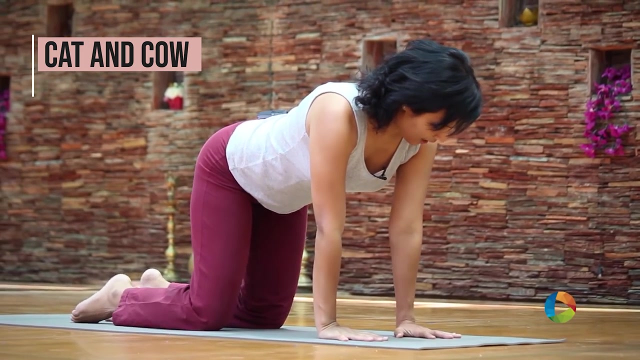 Drop them back in your heart. Okay, Down. Now the same thing again. Join your legs together From a comfortable sitting posture, come into the box position, Hit the wrist directly under the shoulders, The knees in line with the palms, Directly. 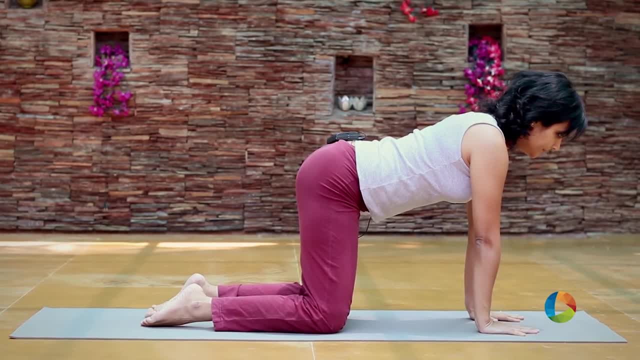 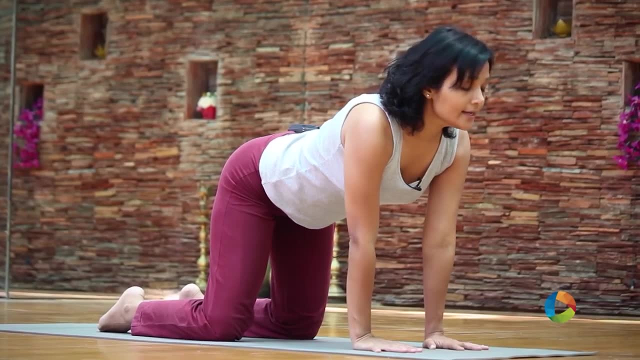 under the hip. The movement is only in the back and not in the limbs. As you inhale, you drop the back down, The head up. Exhale, you arch your back up. Look at your knees- Inhale- 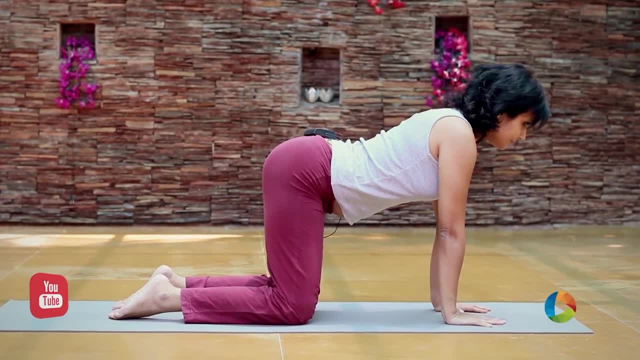 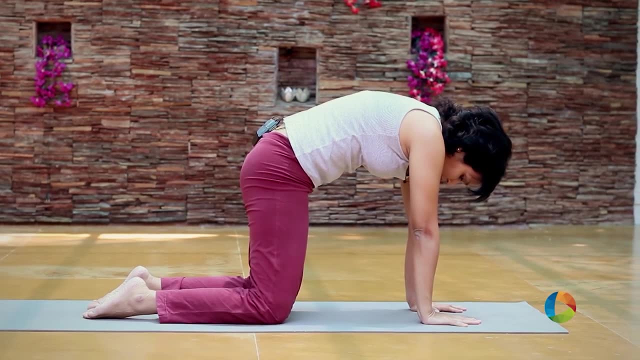 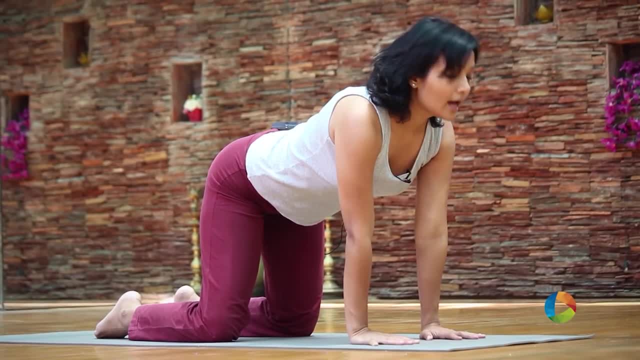 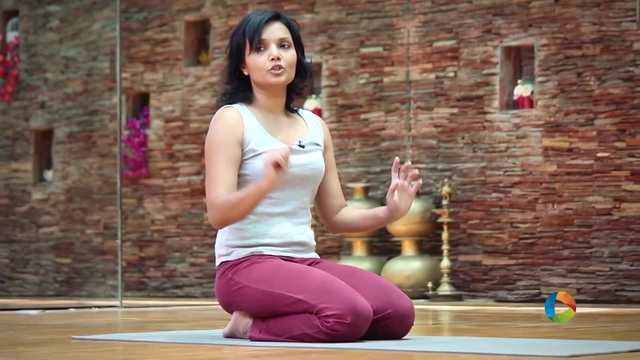 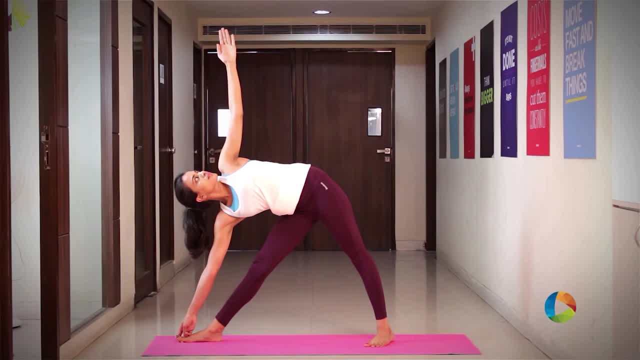 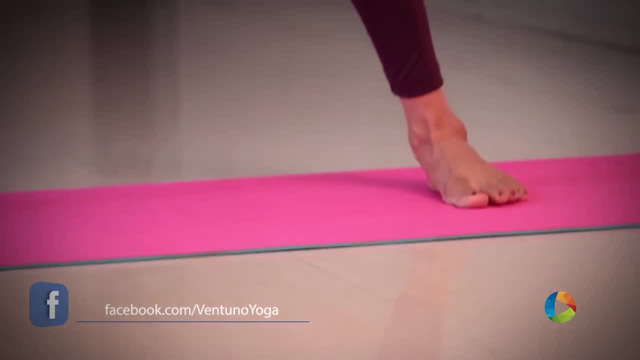 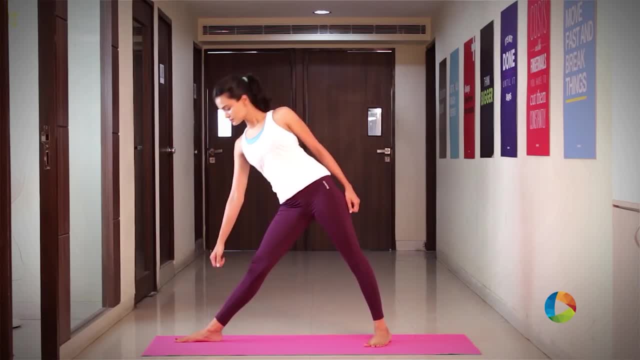 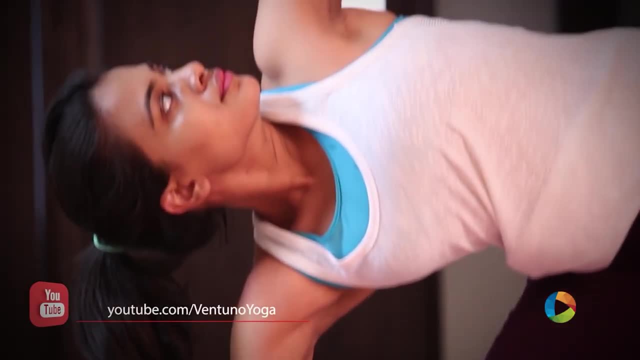 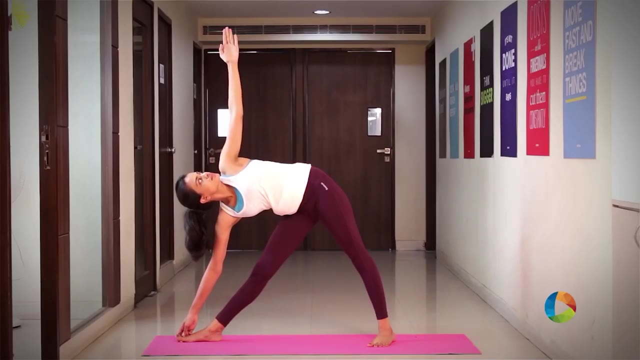 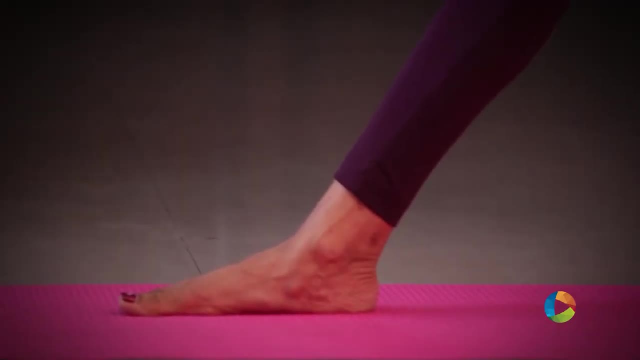 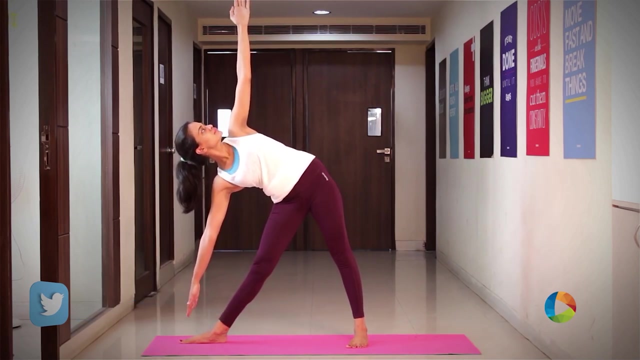 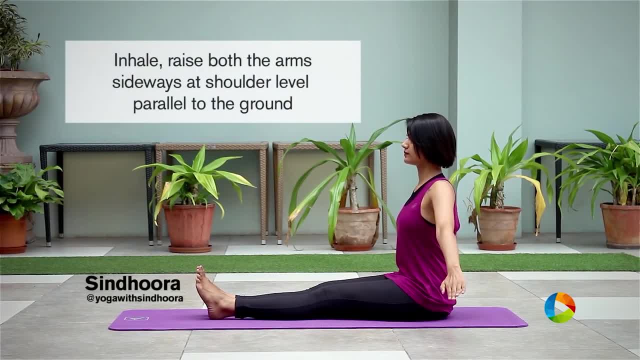 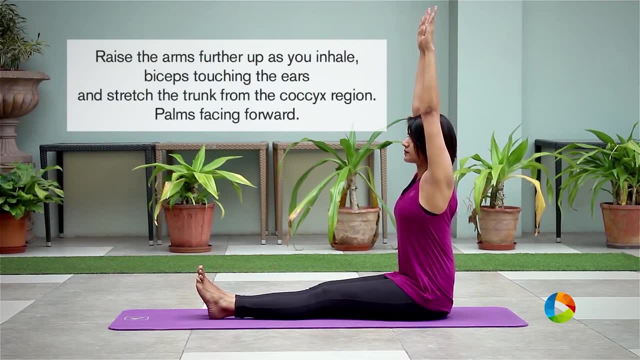 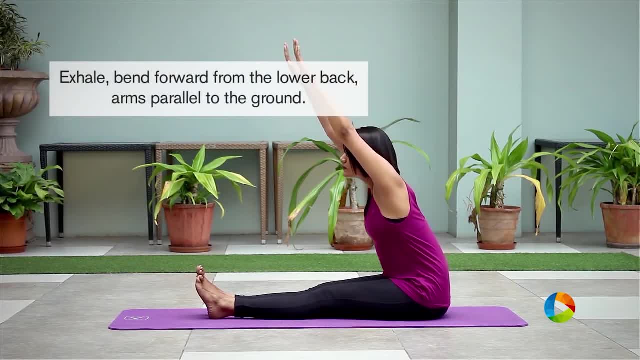 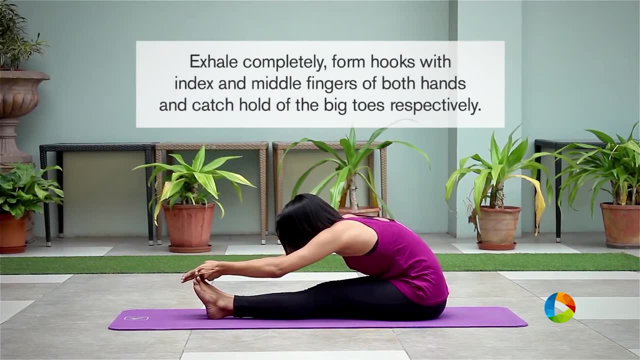 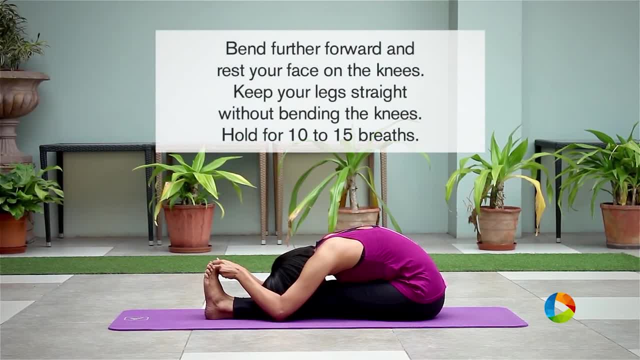 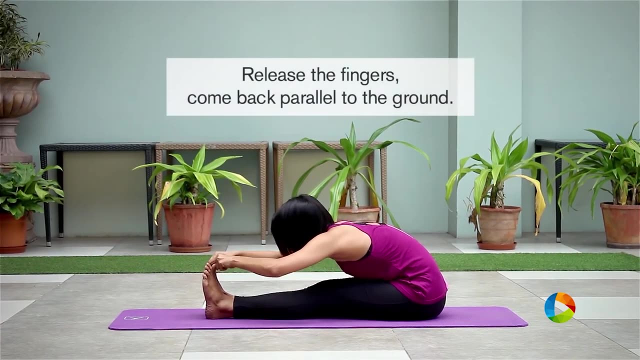 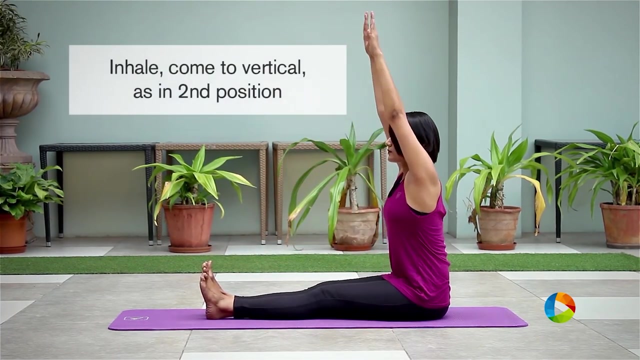 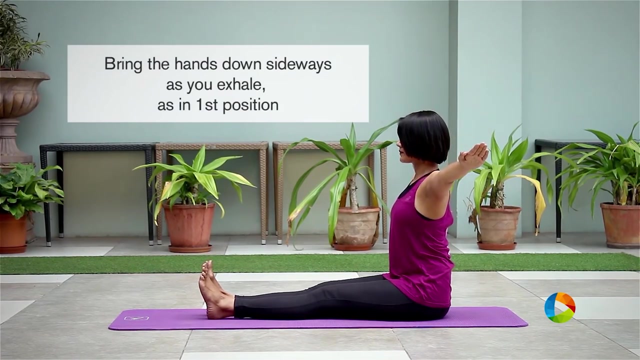 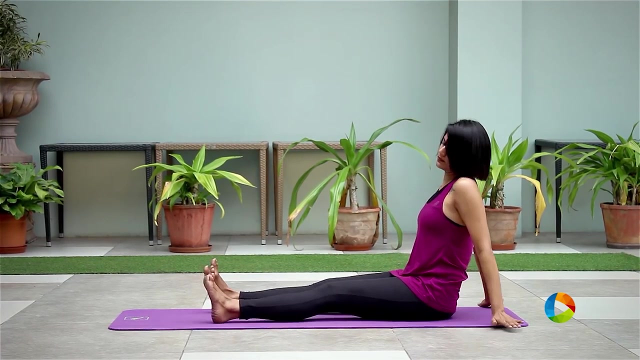 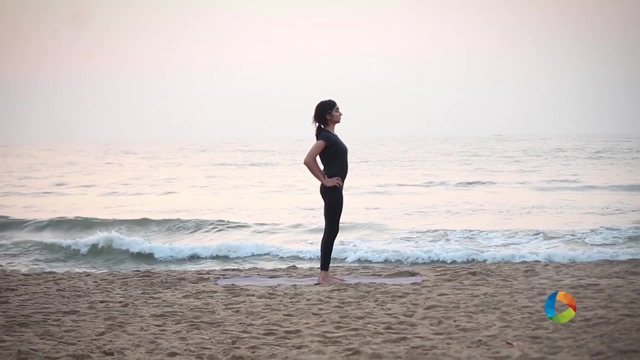 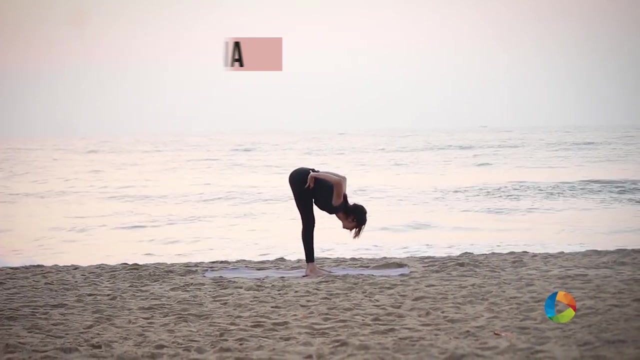 exhale, exhale, Thank you. Keep your feet hip distance apart. Inhale, breathe through the chest. lengthen the spine. Exhale slowly with control. bring your head down Now. grab hold of the toes with the middle index and thumb. 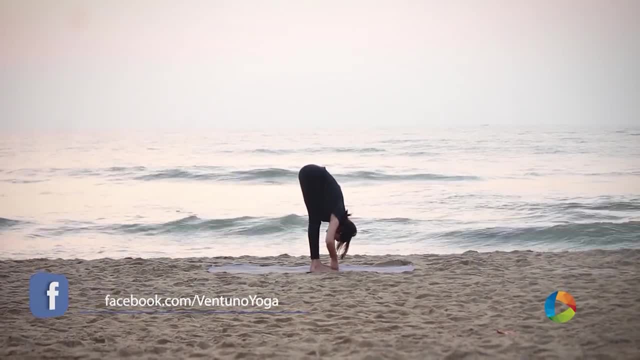 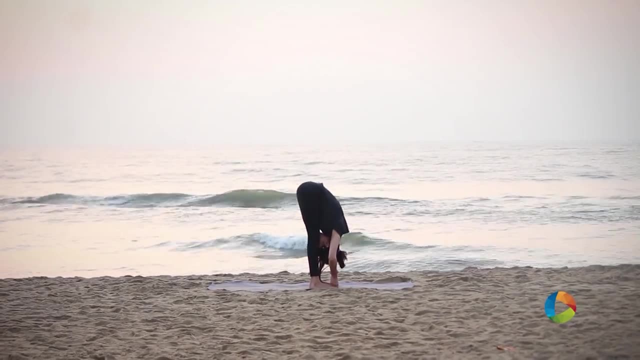 Inhale- lift the chest. Inhale, lengthen the spine. Exhale- bring your forehead down Padangusthasana. Take slow five deep breaths here. Inhale- lengthen the spine. breathe through the chest.